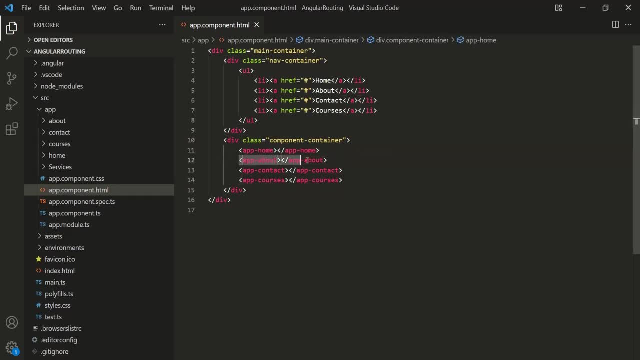 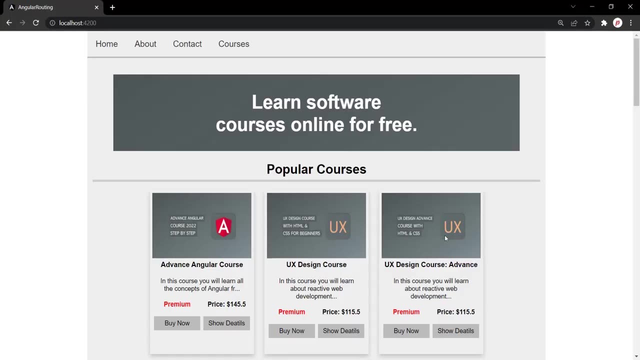 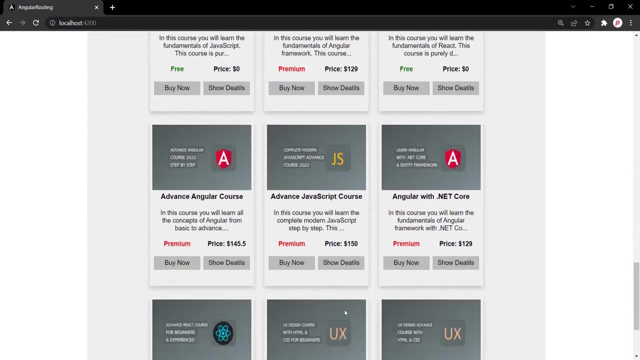 And inside this div we are using the selector for home component, about component, contact component and courses component, And that's why in the webpage you will see that the view of each of those components are being displayed here in this webpage, Okay, And in this app component. 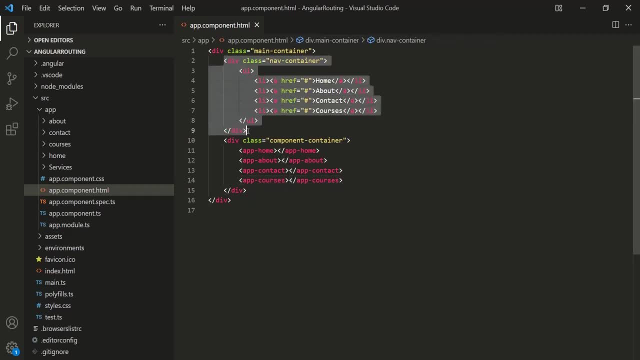 I have also defined a navigation bar. So here, using this div, we are creating a navigation bar And inside this navigation bar we have defined four links: A link for home page, a link for about page, a link for contact and a link for courses. Okay, And that's what you will see in the webpage. 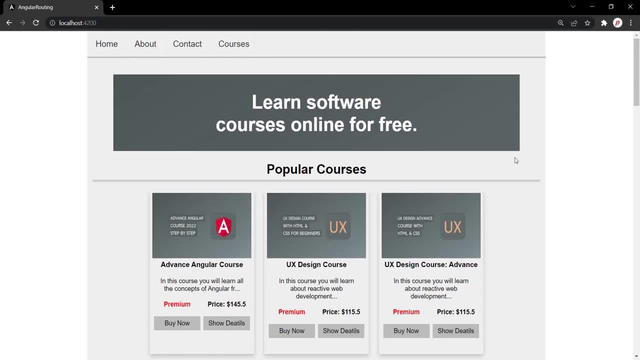 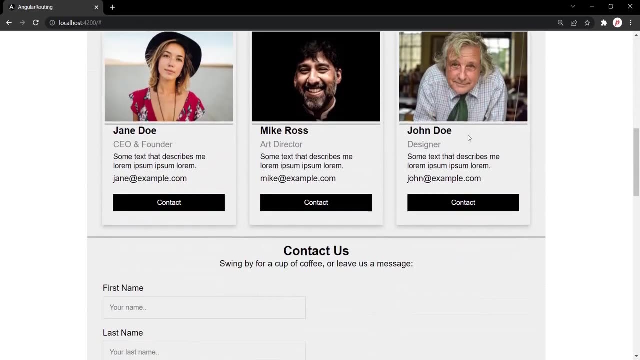 Now, instead of displaying the view of each of these components in the same page, we want to display only that view for which the user has clicked the link. So, for example, if the user has clicked this contact link, in that case we only want to display the view of that contact. 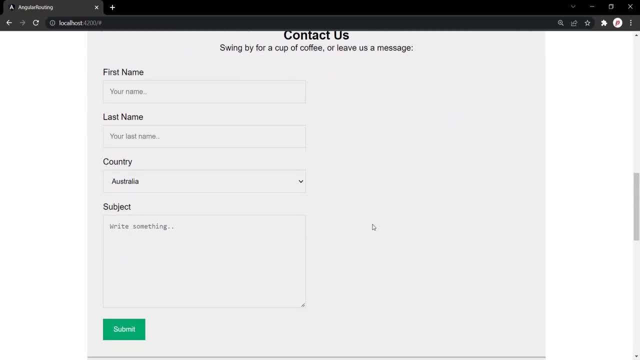 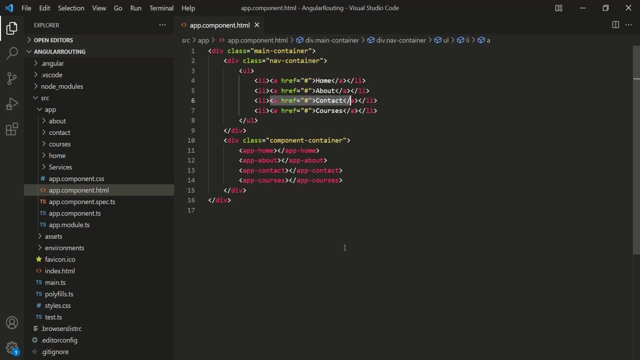 page. Okay, So this view. For that we can use routing. So let's see how to implement routing in Angular. Let's go to VS code Now. we can create routes in a separate TypeScript file or inside AppModules, And I am going to create routes for this Angular application inside the 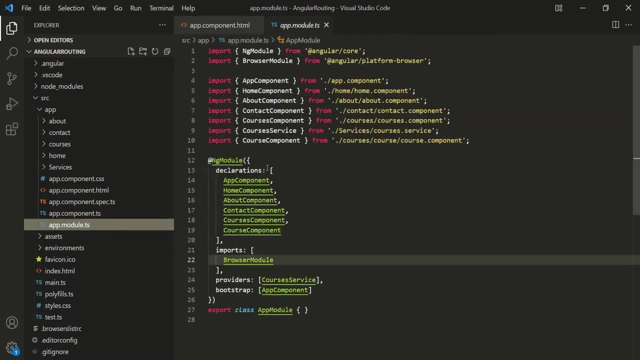 AppModules file. let's open this appmodulests file and before this ng module, let's create a constant using this const keyword and let's call it app route. and you can name this variable anything, but the type of this variable should be routes. Okay, it should be routes and not route, and in: 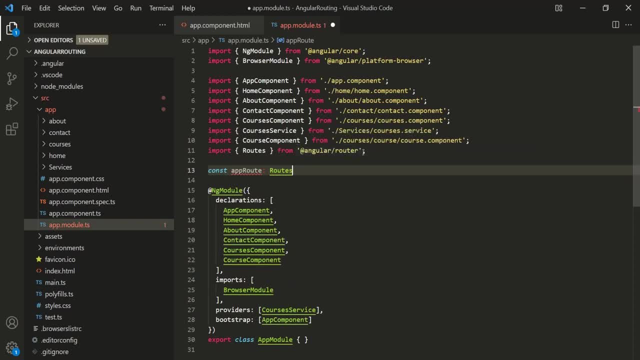 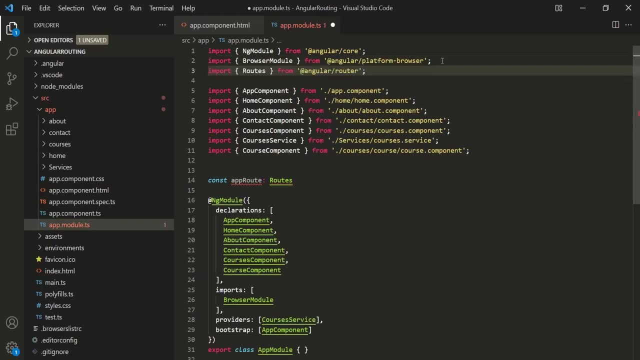 order to use this routes, we also need to import it from angular slash router. Now, let me move this import statement at the top, So I'll cut it from here and I'll use it here. Now, if I hover over this routes, you will notice that this routes is an array of route objects. Okay, so to this. 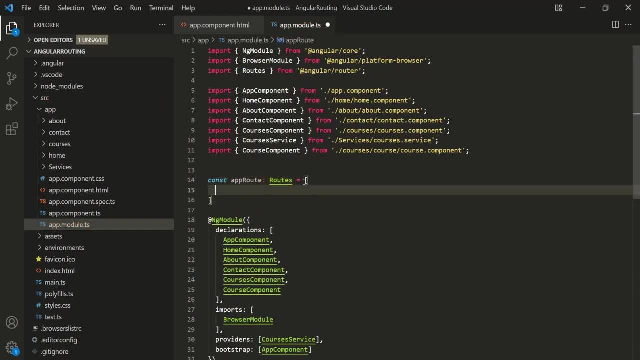 we can assign an array and inside this array we specify the route, objects For that. we use this object, literal syntax, and inside this object, literal syntax. we specify this object, literal syntax, and inside this object, literal syntax. we specify this object, literal syntax, and inside this object, literal syntax. we specify this object literal syntax, and inside this: 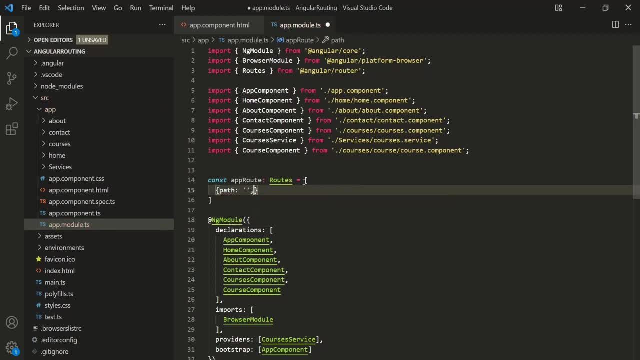 object literal syntax and inside this object literal syntax, we specify this object literal syntax and inside this object literal syntax and inside this object literal syntax, we specify the path property which is of type string, and we also specify the component property and to this component property we can assign a component class, For example home component. about component. 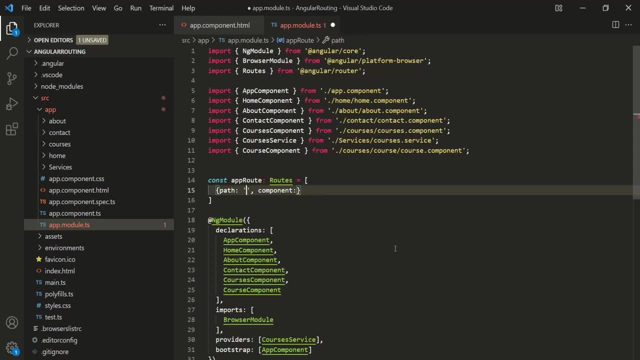 etc. Okay, so what we want is when a user types route URL, slash home in the address bar. in that case we want to render the view template of home component. So to the path, we have assigned this path home, and when this path is typed in the url, we want to render the view template of home. 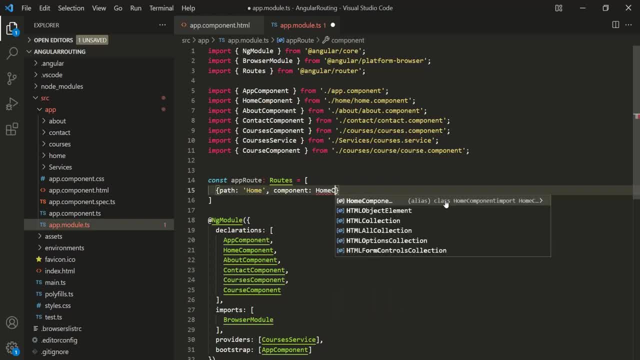 component. so to this component property we can assign home component class and in this way we have created one route. in the same way, if a user types root url, slash about in the address bar, so here the path will be about in that case. i want to render the view of about component. 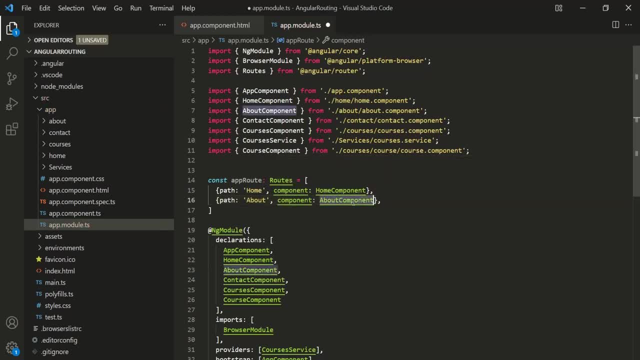 so to this component property we can assign this about component class. okay. in the same way, let's also go ahead and create routes for contact and courses. so here let's specify the path as contact and, and when this path is typed in the url we want to display the view of contact component and in the 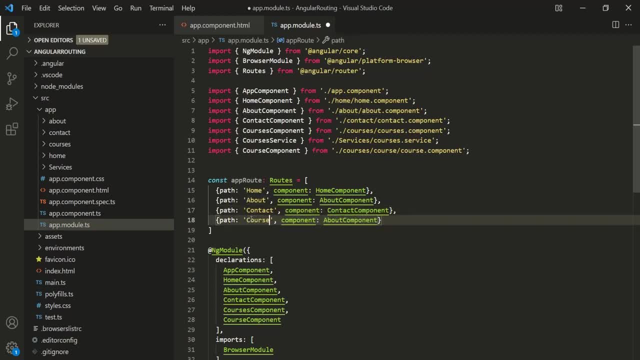 same way, let's also specify a path of courses and when this path is typed in the url, we want to display the view of courses component. okay, so in this way we have defined four routes, but our angular application does not know about these routes yet. so to make this application know about 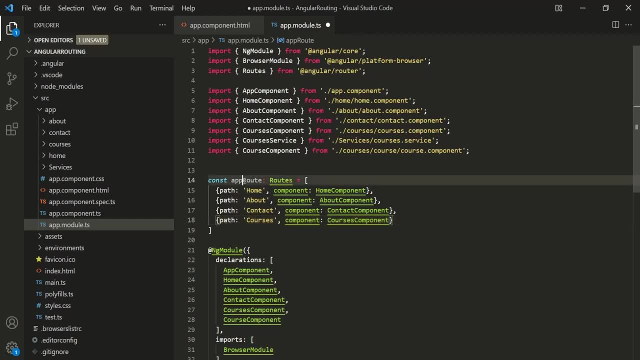 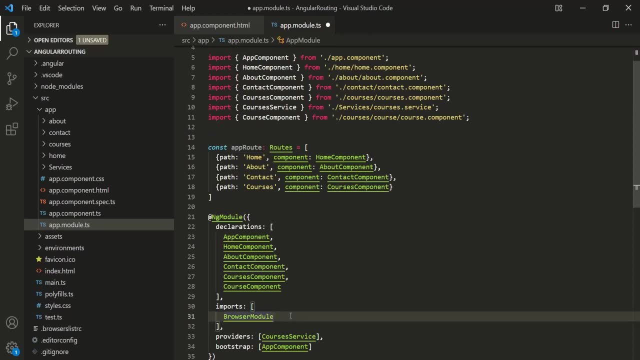 these routing steps. so if we want to use these routes, we need to register this app route and to do that, in this imports array we need to add router module. so let's do that. so router module. and in order to use this router module, we also need to import it from angular. slash router. now, on this router module we can call a method called for root, and to this for root method, we can pass out route interface from rectangular to center. so this will be legible in ourhehe. now let us look at the other side of the. 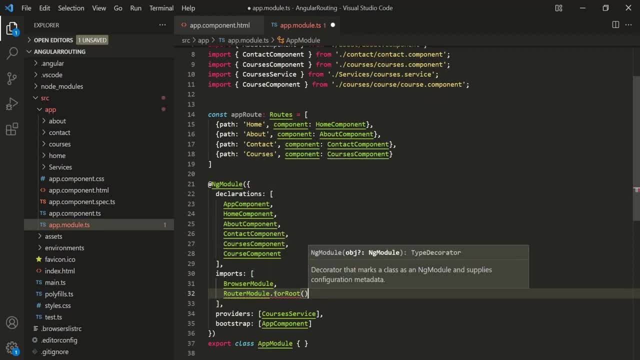 eeth logic here. now in this flavor we can have input request option where we need to use ingratiator. now on this router module we can call a method called for root and to this for root method we can pass out active democratic. to this for root method we can pass out active innovative software. for this we can condition EIXor for rootINTиюmeral. 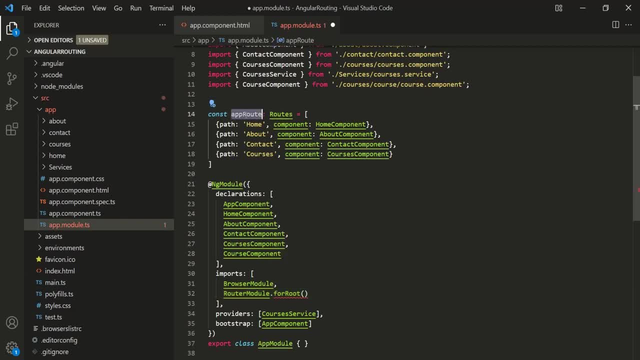 method we can pass our route, so we are storing our route inside this app, route constant. let's pass this to this for root method and with this, this angular application knows about these routes. finally, we need to tell angular where to display the view when one of these paths are typed in the 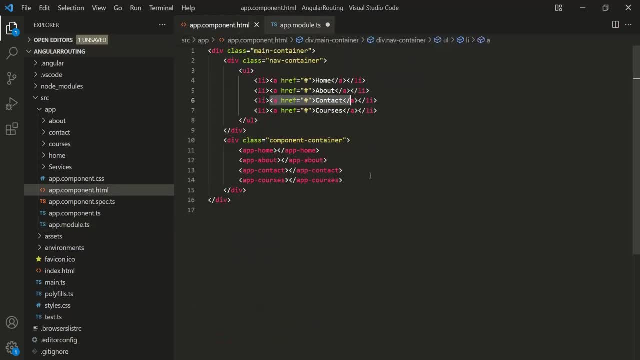 url. so in this case we want to display the view inside this div which we have created inside the app component dot html. so from here let me comment these selectors: okay, and here we can use a directive which is router hyphen outlet. so this router outlet is a directive that tells angular 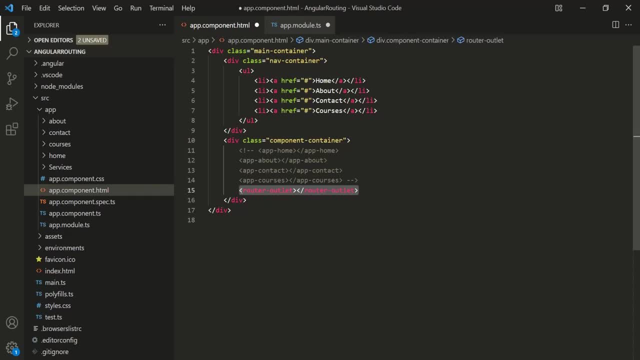 where in our page we want to display the view and we do not have to imagine that we have to display the view. we do not have to imagine that we have to display the view. import this directive. that's because this directive is imported. when we imported the 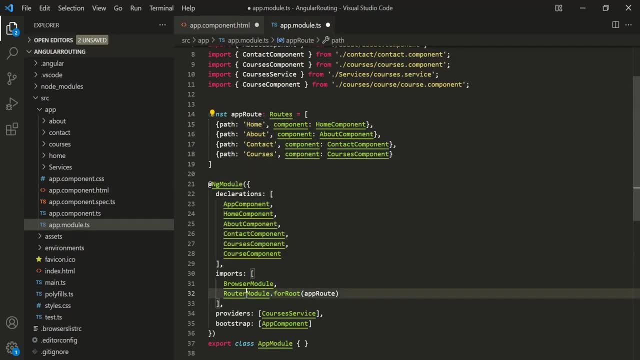 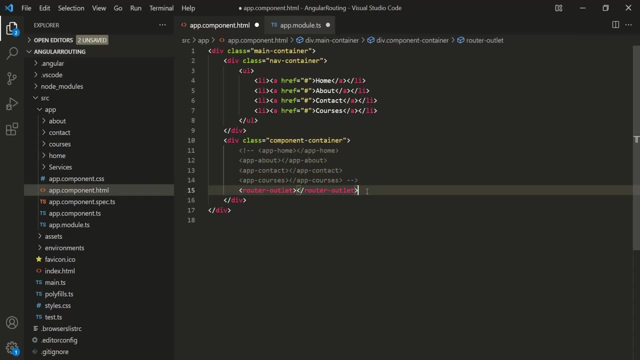 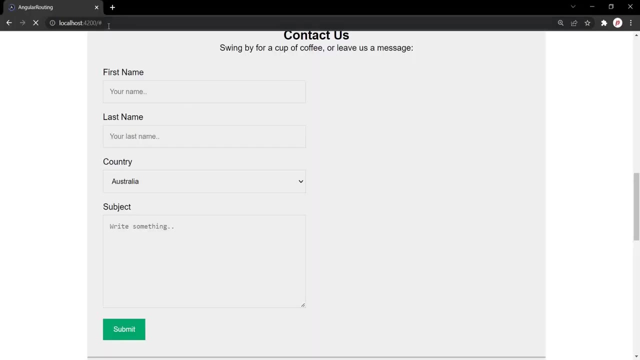 router module in our app modules file. so when we imported this router module here, with this this directive also get imported. okay, and with this the routes should be working now. so let's save the changes, let's go to the web page and so you can see: for the root url, no content is. 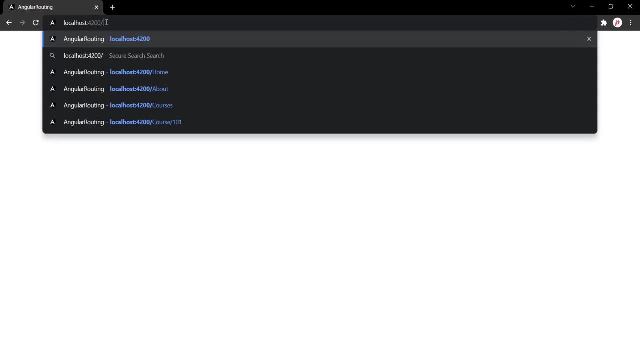 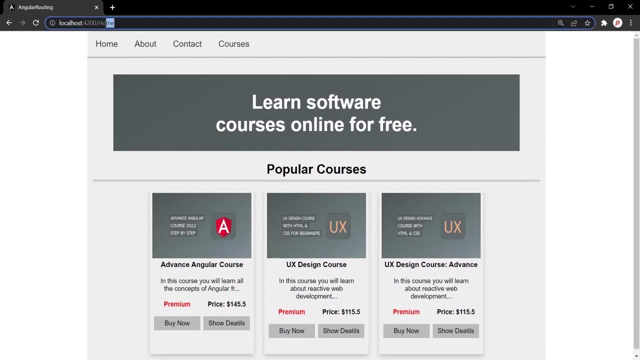 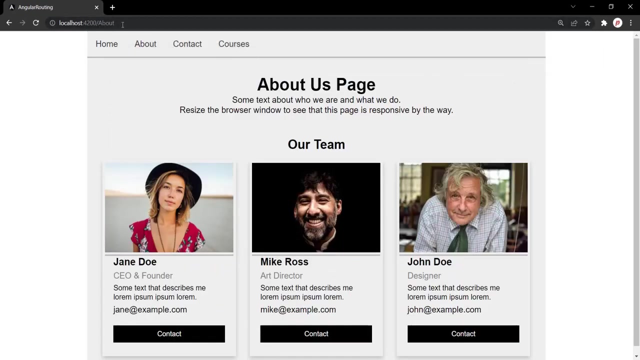 being displayed. okay, now let's type root url- slash- home, press enter, and it is displaying the view of home component. now let's type root url- slash about, and now it is displaying the view of about component. so in the route you can see that when in the url the user types this path, 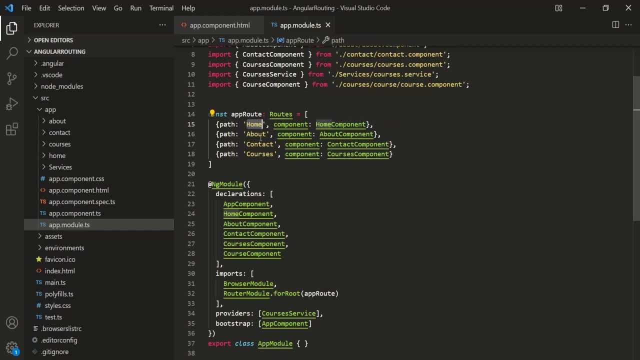 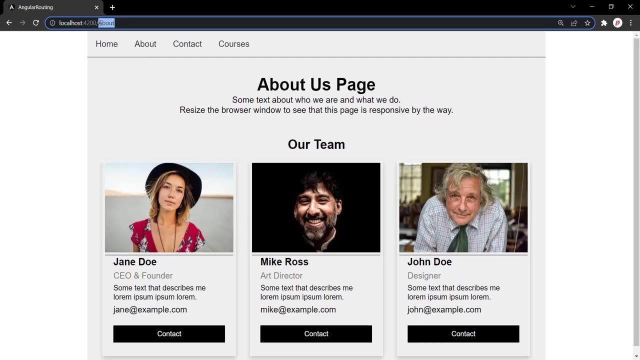 home, then it will display the view template of home component. in the same way, when the user types you this path in the url- so root url slash about- it will display the view of about component and that's what you're seeing in the web page. in the same way, if i type the path has root url slash. 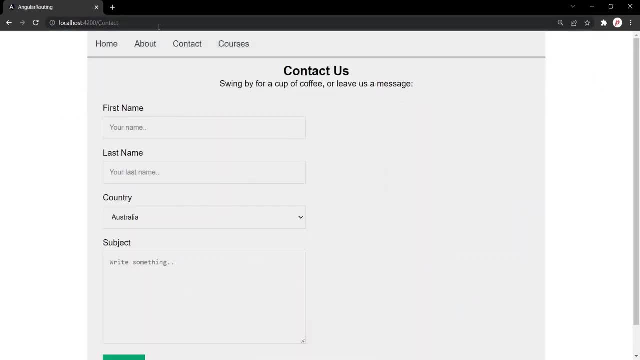 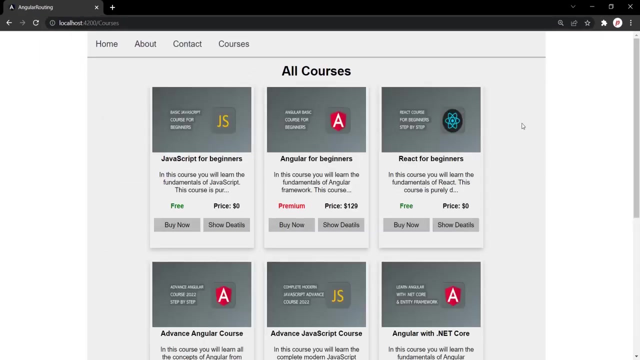 contact and press enter, it will display the view of contact component. and finally, let's also type the path for courses. okay, so when i press enter now it is displaying the view of courses component. so our routes are working as expected. but here we have one bug. so the bug is: if i remove 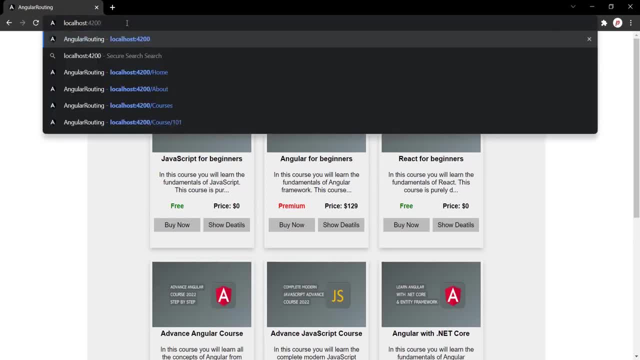 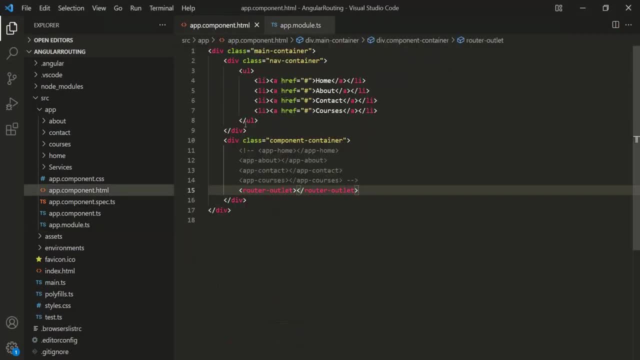 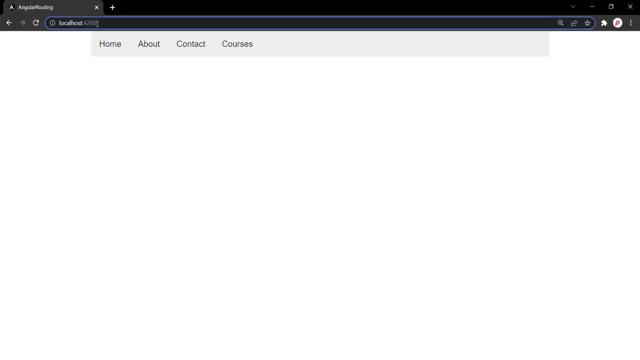 these paths from here, and if i only type the root url and press inter, in that case it is only displaying the navigation bar. so it is only displaying this navigation bar and it is not displaying any other content. that's because for this url, this localhost, column 4200. 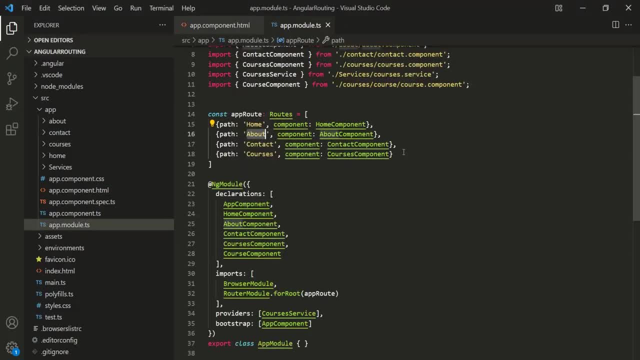 we have not defined any route inside this routes array, so let's define a route for the root url. so again, let's use this object, literal syntax, and for the root url the path will be empty string. okay, and let's say, when the user types the root url in the url bar, in the address bar, we want to. 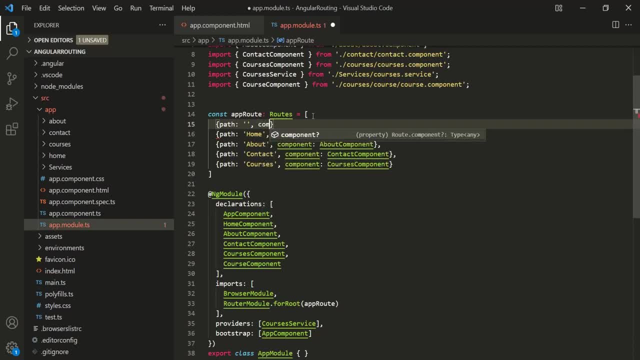 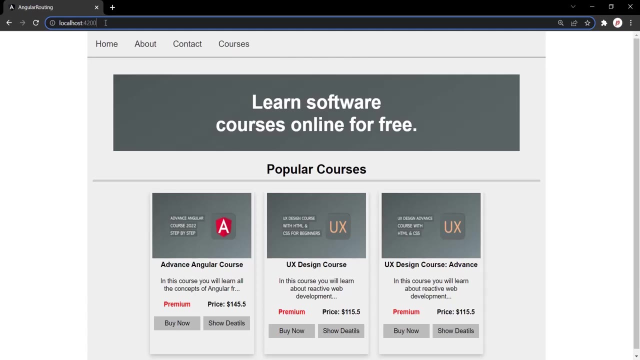 display the view of home component. so to this component we can assign this home component class. okay, with this, let's save the changes. let's go to the web page and now, when i type the root url and press enter, the view of home component is being displayed. okay, so it is working as expected. 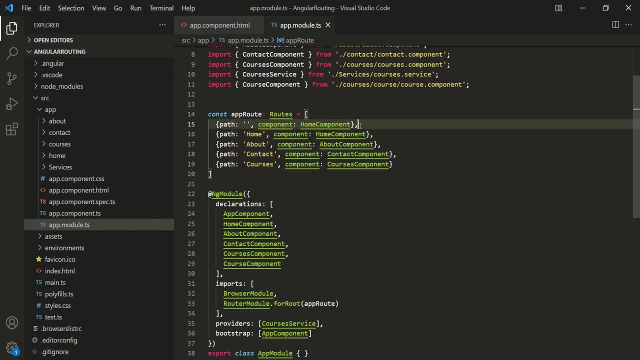 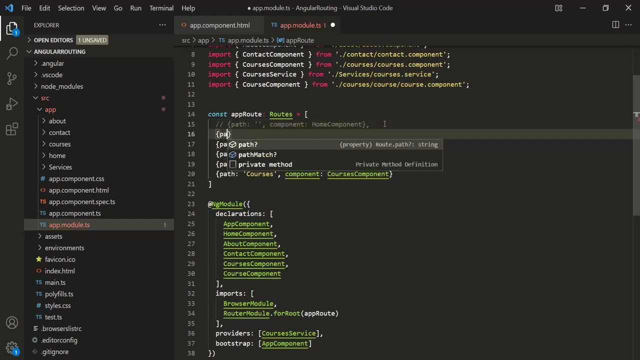 so this is one way of defining a route for the root url, and this route, the route which we define for the root url, is called as default route. so this is one way of defining a default route. another way is- so let me comment this line and let's again use an object literal syntax here- so another way is we can specify the path as: 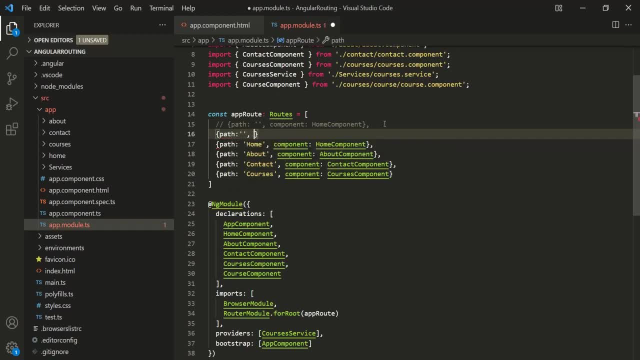 empty string for the root url, then we can use another property which is redirect to and to this we can specify the path to which we want to redirect the user when the user enters the root url. so here, when the user enters the root url, we want to redirect him to the home page. 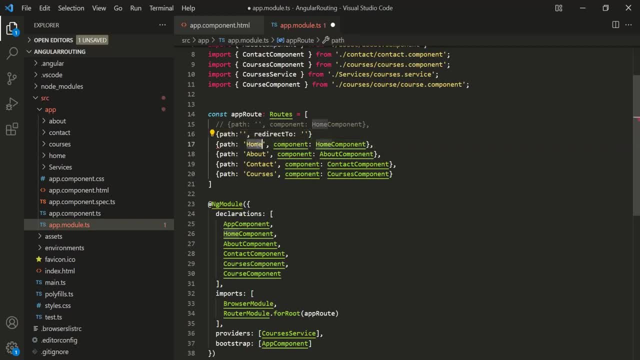 so to this, redirect to. we can specify this path, this home, so let's specify that, okay. and finally, we also need to specify a property called path match and we need to set it to full, and this should be path match. this path match property simply tells you know, simply tells the router how to match the url. 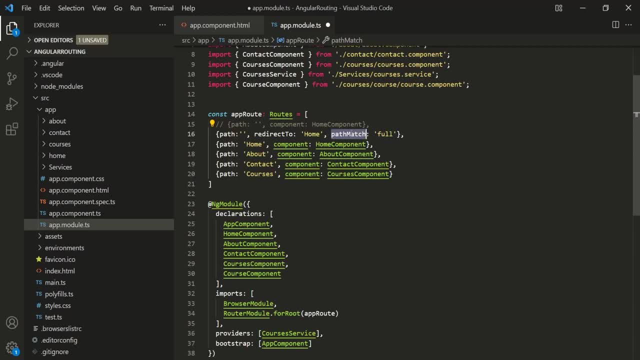 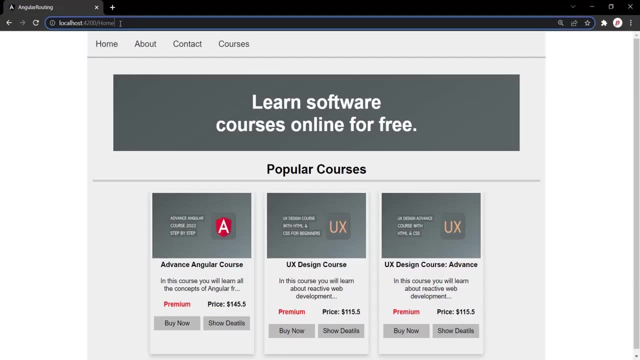 and when it is set to full, the path is matched to the entire url. with this, let's save the changes. let's go to the web page again and still, when i enter this root url and when i press enter, you will notice that we are redirected to. 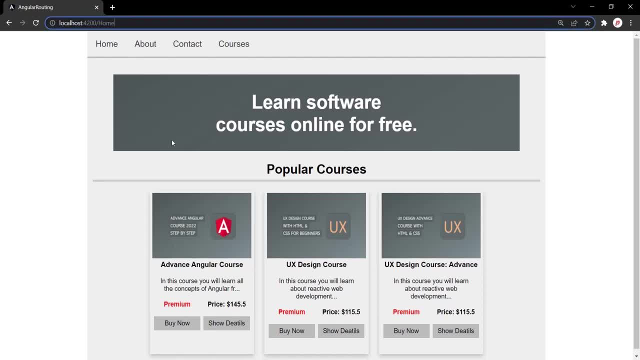 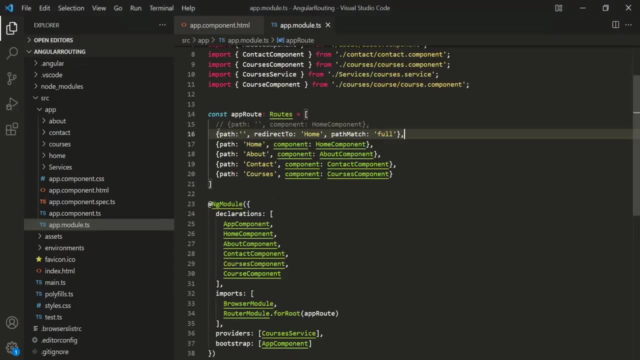 root url slash home. okay, and it is displaying the view of home page- okay. so even if i enter root url here and press enter, it will redirect us to root url slash home. but if we use this approach, so if i comment this and uncomment this route, if i save the changes, in that case there will 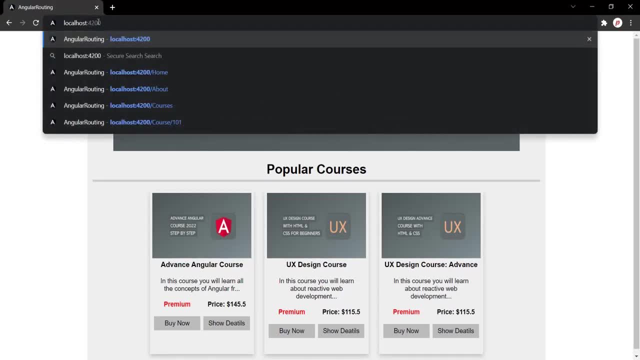 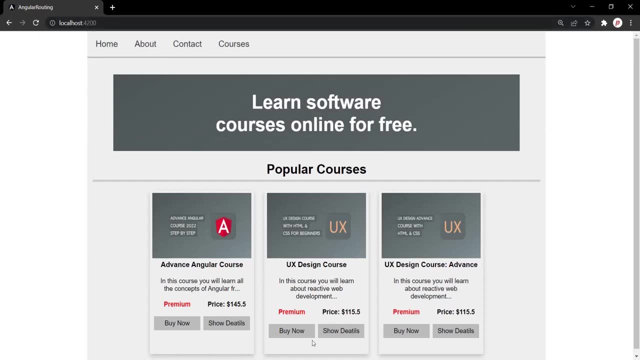 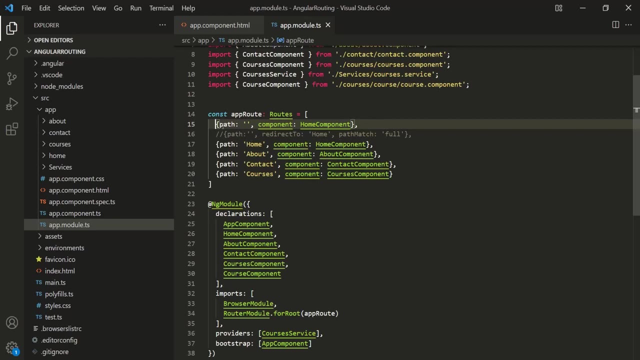 there will be no redirection. okay, so if i type root url and press enter, we are still in that url and it is displaying the view of home component. so that's the difference here. in this case, there will be no redirection happening. but if we use this approach, in that case we will be.